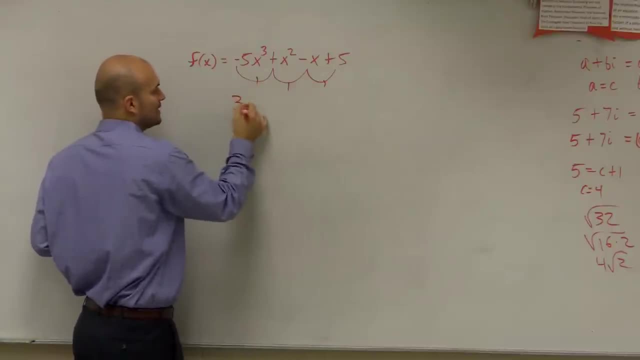 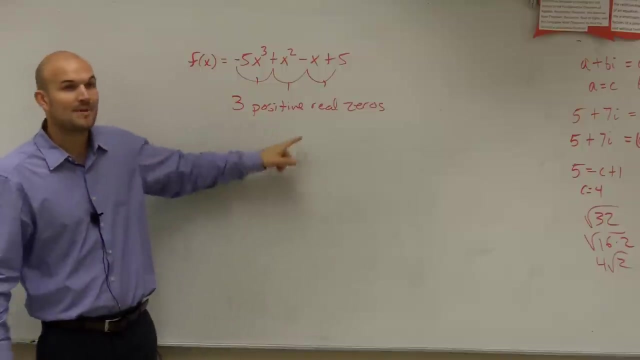 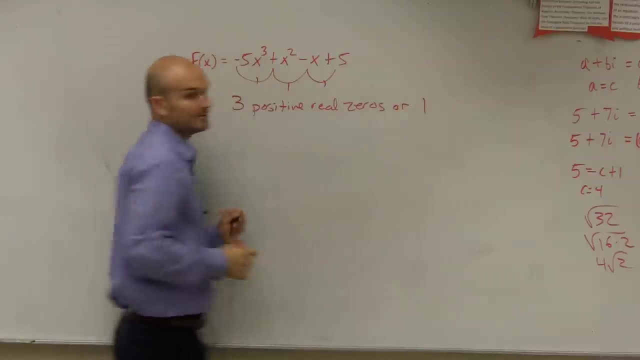 Yes. So therefore I have a possible of three positive real zeros. Now remember, this is only talking about real zeros. all right, Real zeros, not imaginary real. So therefore I have three positive real zeros, or minus that by an even integer or 1.. So you take 3 and then subtract 2, which would be your even integer 1.. Or it could be if you. 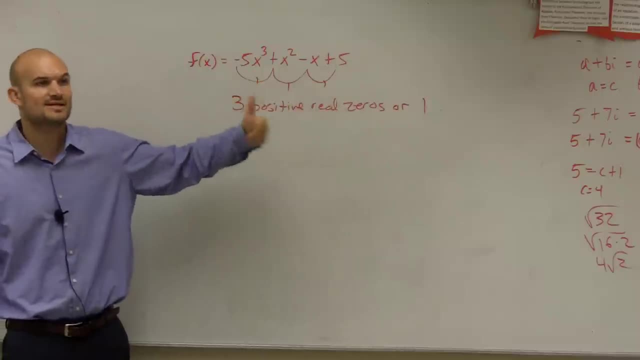 If you have multiple, it can keep on going down. Let's say you had 6. It could be 6,, 4,, 2, or 0. So I have either 3 positive real zeros or 1 positive real zero. 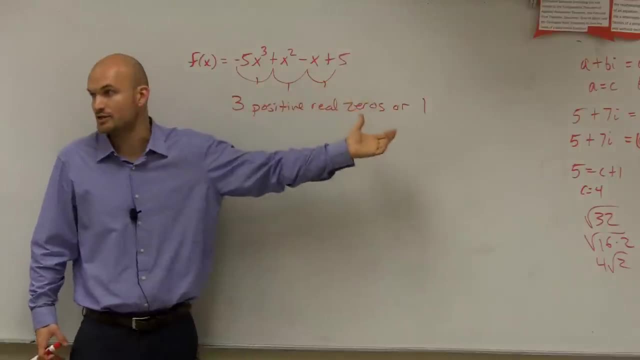 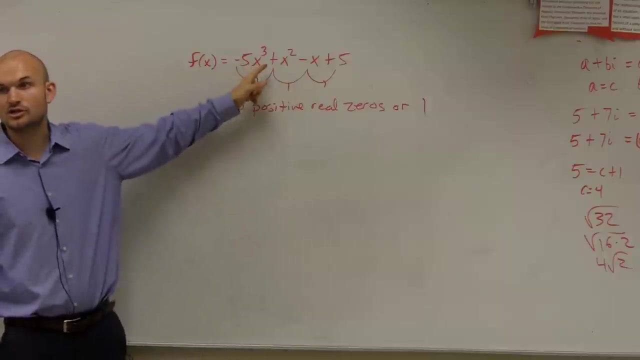 So you take the number of variations and then subtract it by your even integer. Now that's for real zeros. If you guys look at this, f of x equals x cubed, My linear factors, how many possible zeros do I have, real and complex? 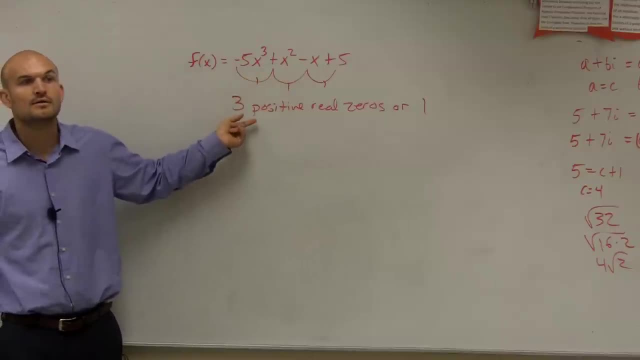 Three. So is it possible for all my zeros to be positive? Yes, right. Well, let's look at what about the negative. Are there any negative real zeros? So to do that, you're going to do the same test, but you're going to test it for f of negative x. 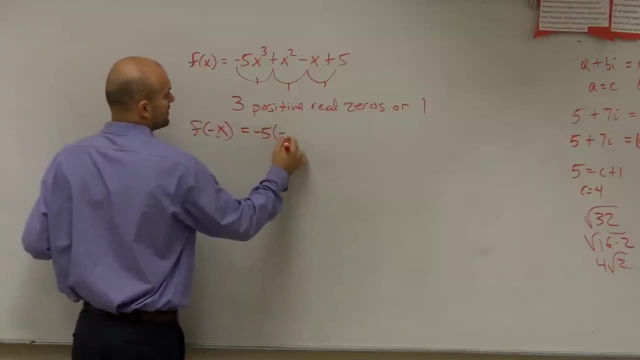 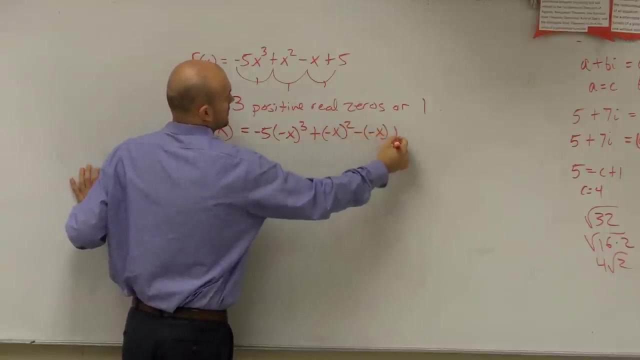 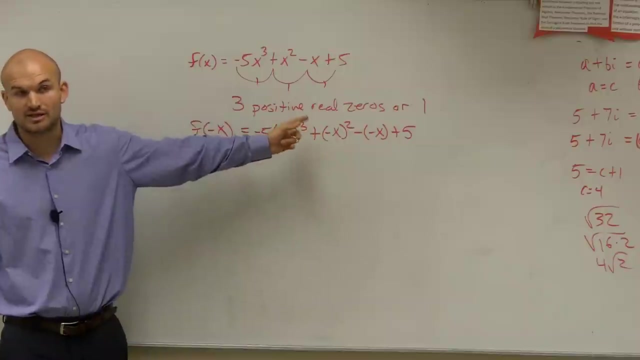 So remember, this is the evaluation tool. So you do negative 5. You plug in negative x. So all I do is, instead of using x, I plug in negative x. Negative x, raised to an odd power, is still going to give me negative x. 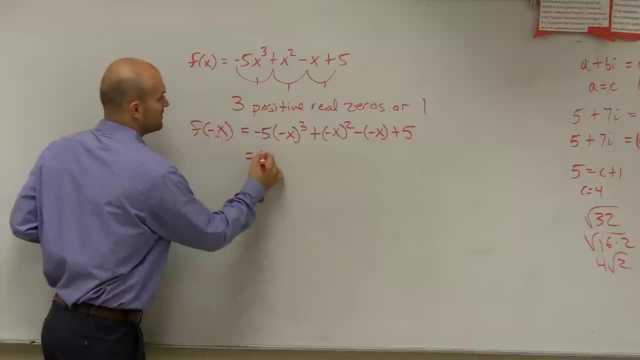 Then times a negative 5 is going to give me a positive 5x cubed, Negative x squared and negative x raised to an even power, which is going to give me now a positive x Squared. negative times negative will be a positive x. 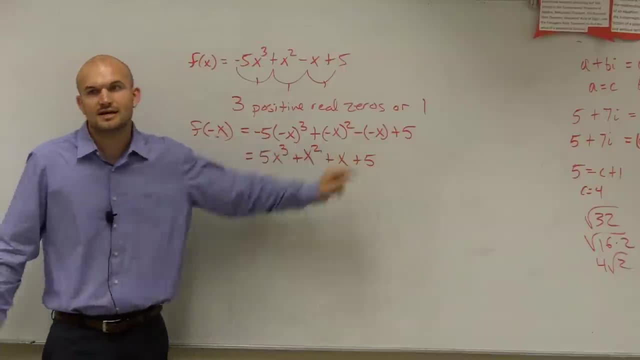 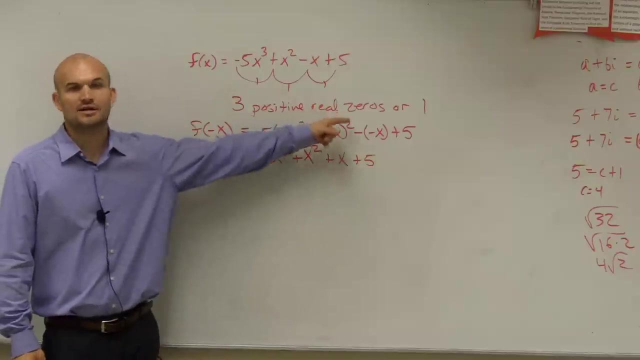 Positive 5.. Do you guys see any variation in sign? No, So. is there any negative real zeros? No, So guess what? All my zeros are going to be positive. So here's why it's helpful If you're going to be doing synthetic division, right? 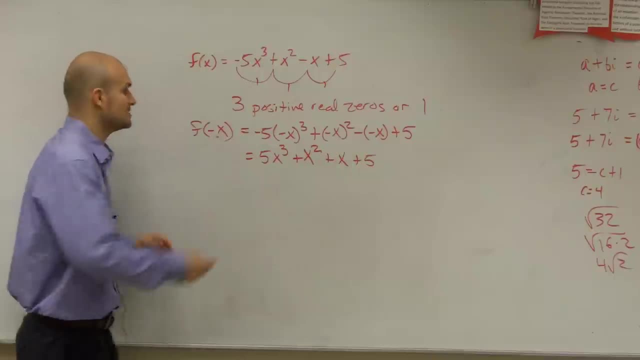 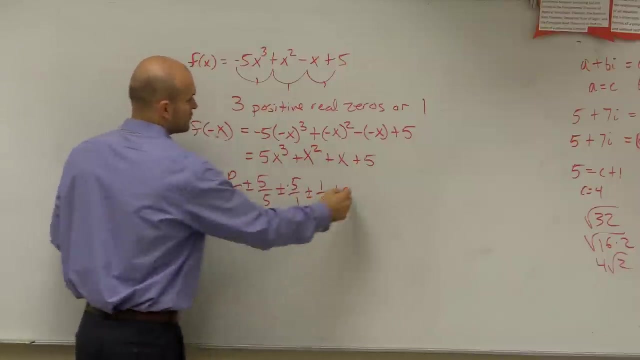 Synthetic division. And let's say you don't have a graphing calculator and you had to do synthetic division By using the rational zero test. you had to do p over q, right? So you're going to do plus or minus 5 over 5, plus or minus 5 over 1, plus or minus 1 over 5, plus or minus 1 over 1, which again is 1..